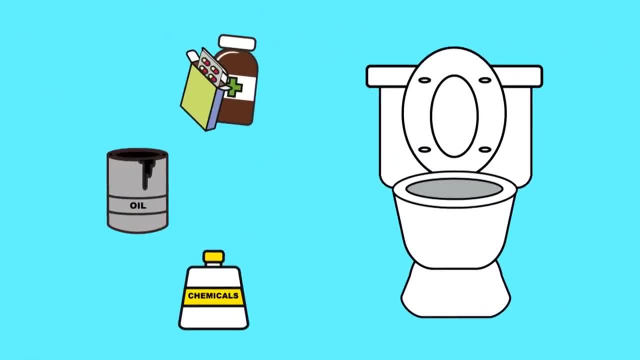 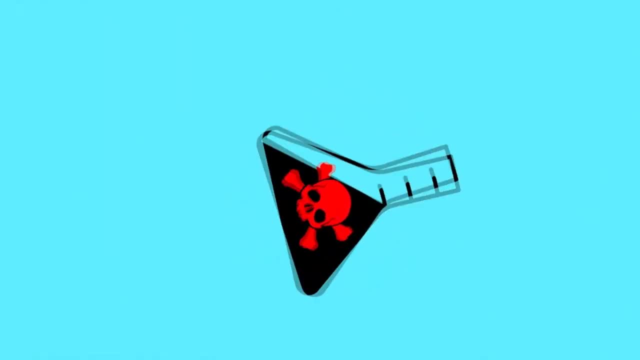 It's important to note that medicines, oil and other chemicals should never be disposed of in the sewage system. Other items are toxic If they are dispersed into the ground through the sewage system or otherwise. they can poison the soil or water and eventually end up in our food. 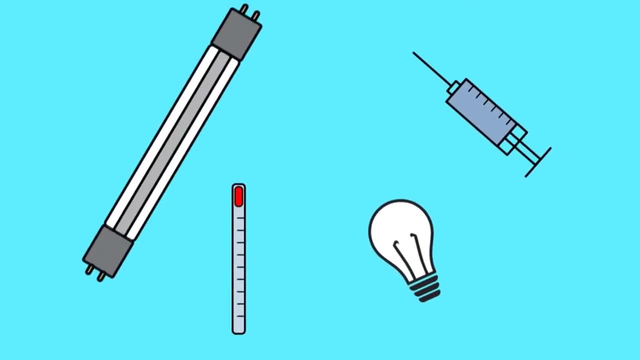 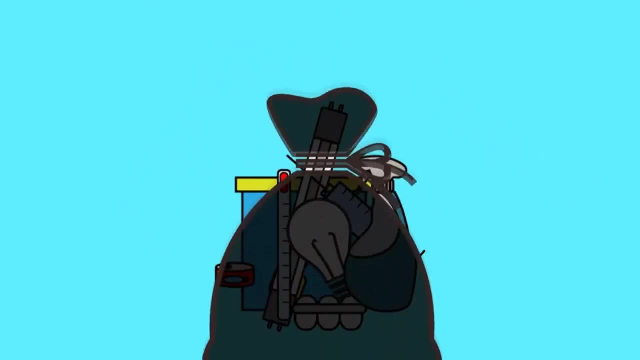 Items such as syringes, thermometers, light bulbs and tubes contain hazardous chemicals. If they are put with other items, they can be very dangerous both to you and the waste handlers. All these types of waste should not be disposed of in the black bag or the recycling. 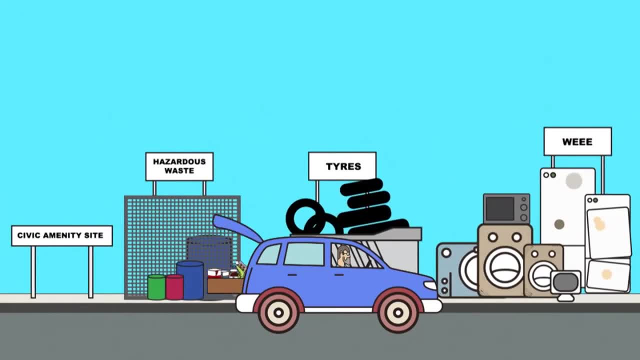 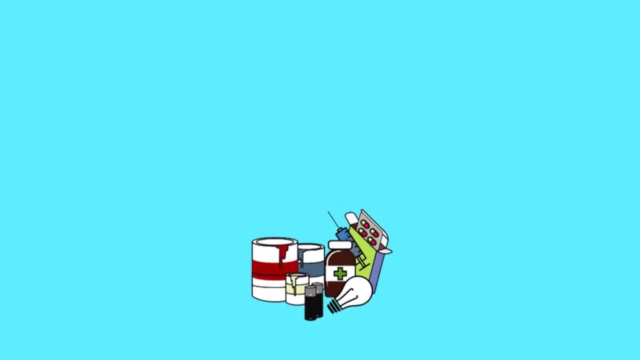 They should be taken to a civic amenity site and disposed of as direct waste. Batteries can also be taken to specific collection points. If disposed of correctly, all hazardous material that cannot be recycled will be disposed of in a controlled manner. With a little effort together, we can reduce the amount of hazardous waste that ends up in the environment. 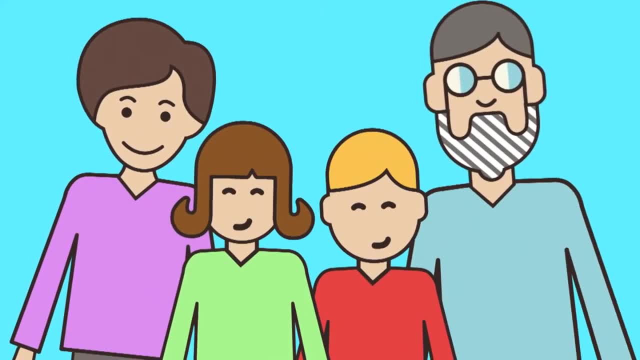 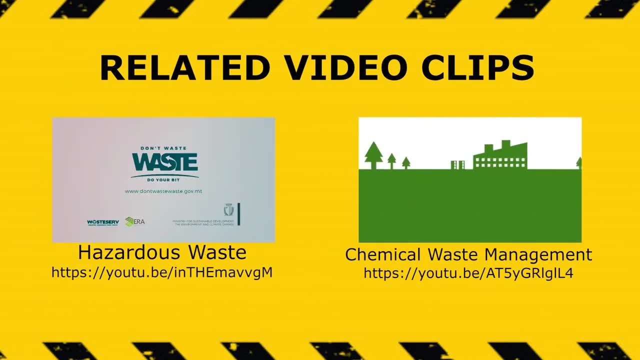 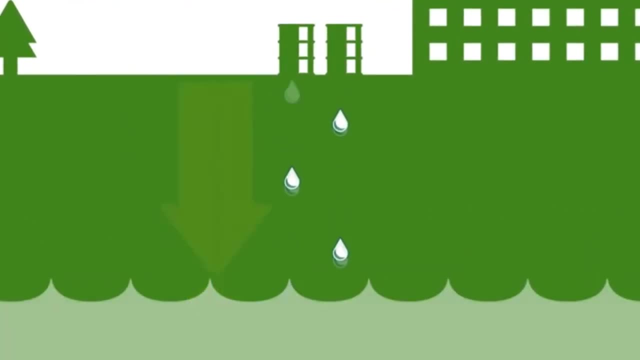 But it's not just better for the environment, It's better for our health too. Don't waste, waste. Do your bit. When hazardous soil and debris goes unchecked in a leachable environment, it can damage the surrounding habitat and even contaminate our groundwater supply. 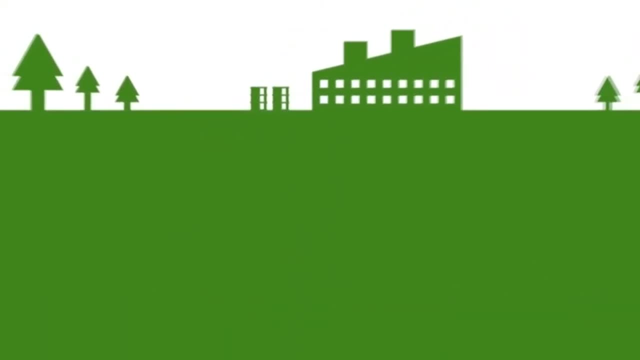 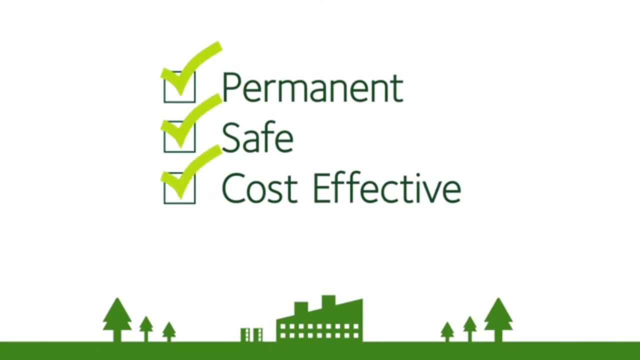 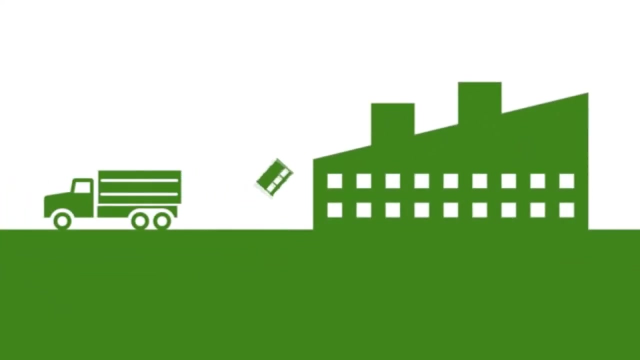 For the benefit of the environment and the protection of our customers. Chemical Waste Management offers a number of innovative hazardous waste treatment methodologies that are permanent, safe, cost-effective and tailored specifically to the type of waste your business generates. Our treatment methodologies help protect the environment from hazardous contaminants and help keep you in compliance. 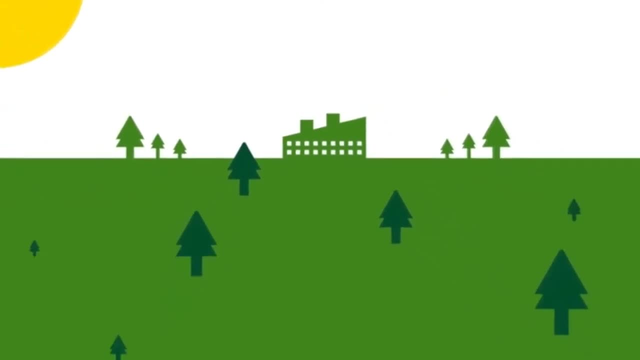 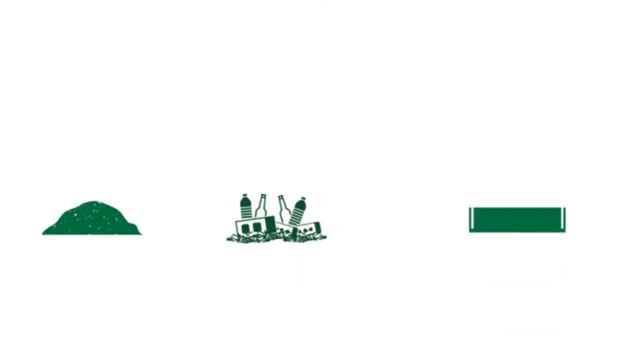 With federal, state and local regulations When it comes to treating hazardous soil, ash, debris and other waste matrices. there are three major treatment methodologies: Stabilization, microencapsulation and macroencapsulation. Each is unique and was developed to address the chemical and physical differences in waste types. 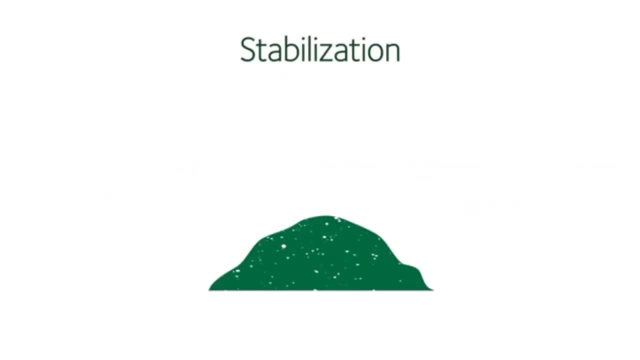 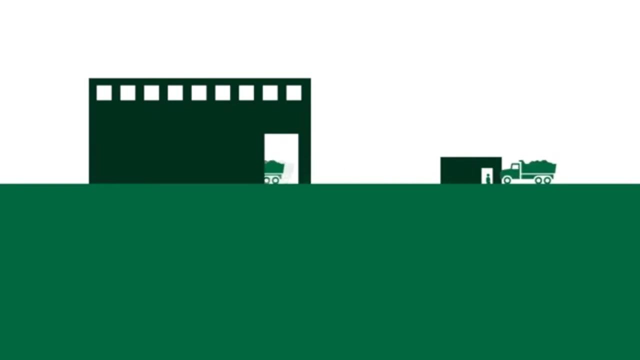 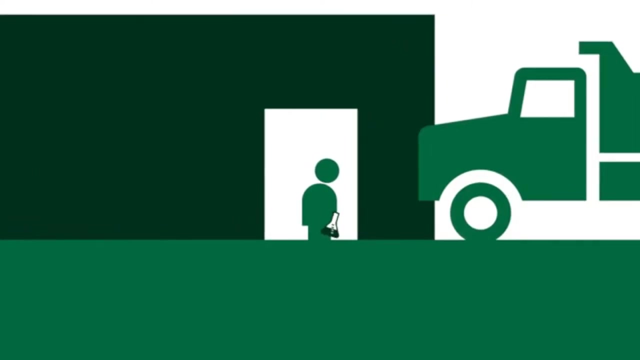 Stabilization is the safest and most effective option for treating soil, gravel, ash and other waste contaminated with heavy metals. If stabilization is determined to be the most appropriate treatment methodology, we develop an empirical formula called the treatment recipe. Once waste arrives at the gate, it is sampled and fingerprinted to confirm if it matches the physical and chemical description before being sent to the stabilization building for treatment. 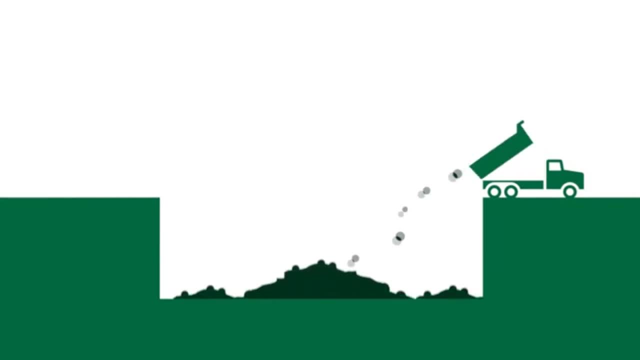 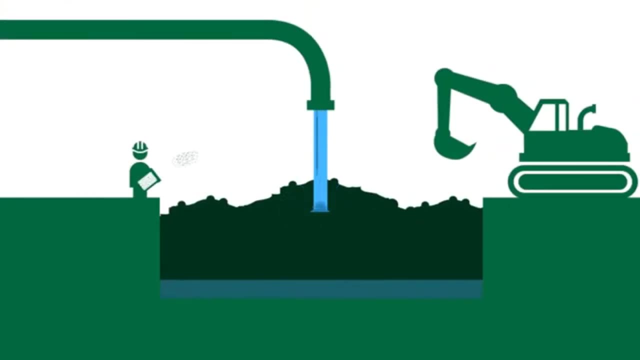 At a dedicated stabilization building. the waste is offloaded into a large receiving and holding treatment unit. Skilled operations personnel add recipe-defined cementitious reagents such as cement kiln dust, POSA, lime fly ash and ferrous sulfate, as well as water, to the contaminated soil. 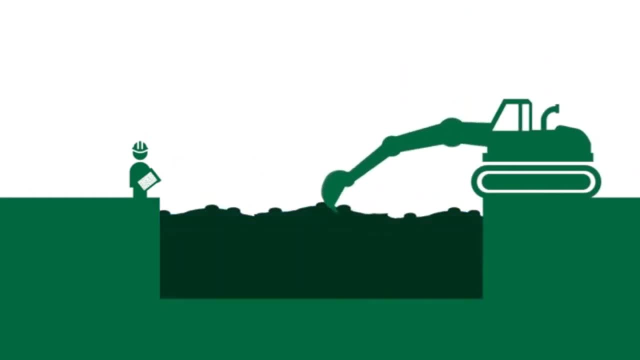 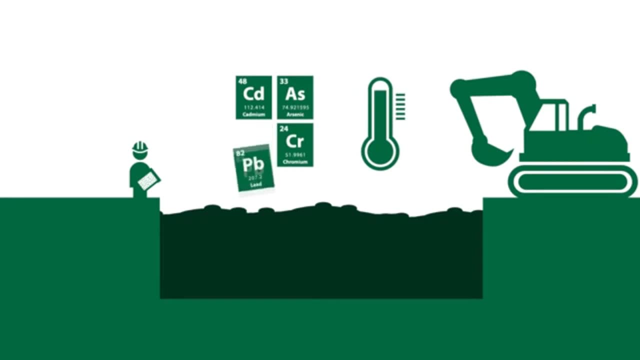 Reagents are mixed by an excavator to begin the process. After the mixture is formed, an exothermic reaction takes place. The reaction binds metal contaminants to the soil, making them less leachable and helping to prevent mobility. The result is a dry, white, dirt-like substance. 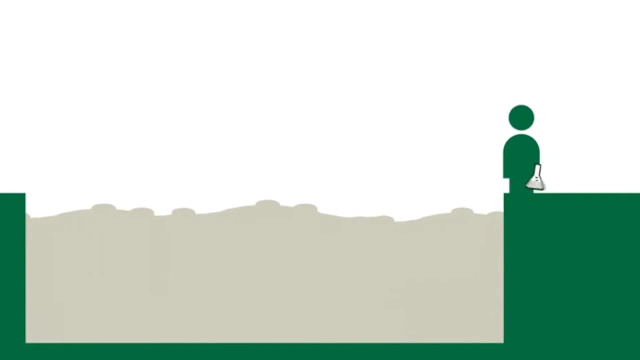 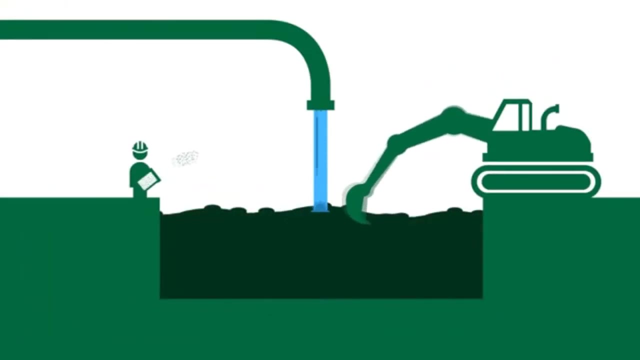 After treatment, the mixture is tested analytically to ensure the process was successful. If the test reveals the resulting mixture does not comply with land disposal restriction regulations, we develop a new treatment recipe and start the process over again After receiving passing laboratory results. 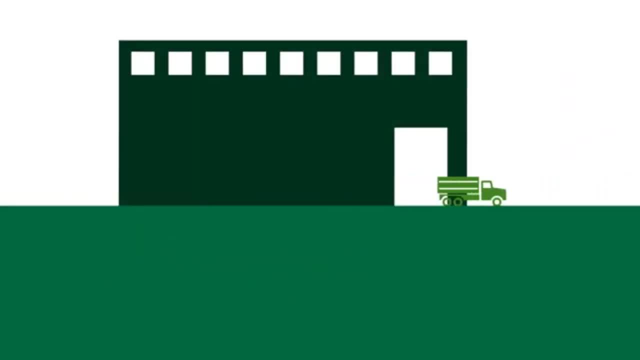 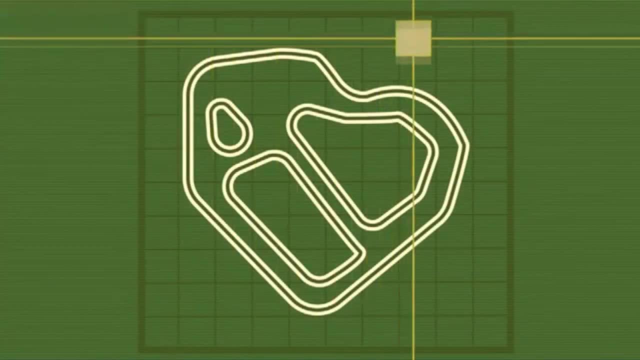 stabilized waste is transported and disposed of at a permitted Subtitle C landfill. to stay compliant with regulations, Treated wastes are placed in a burial cell. Its location is gridded using X- Y Z coordinates, so we know the long-term location of the materials. 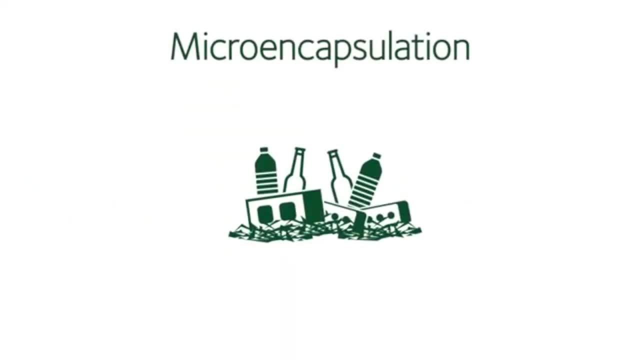 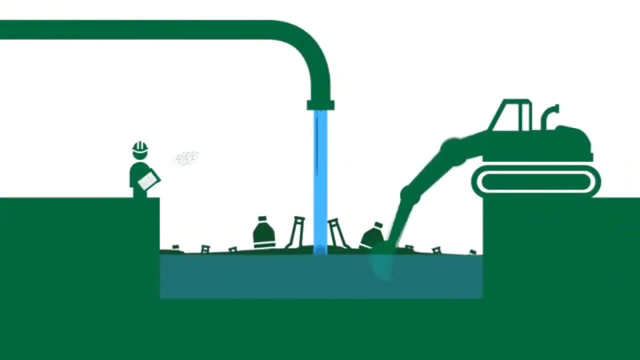 Microencapsulation is similar to stabilization in that the waste is often mixed with reagents such as cement. It even occurs in the same treatment unit, Unlike stabilization. waste types must meet the definition of inorganic solid debris as defined by the Resource Conservation and Recovery Act. 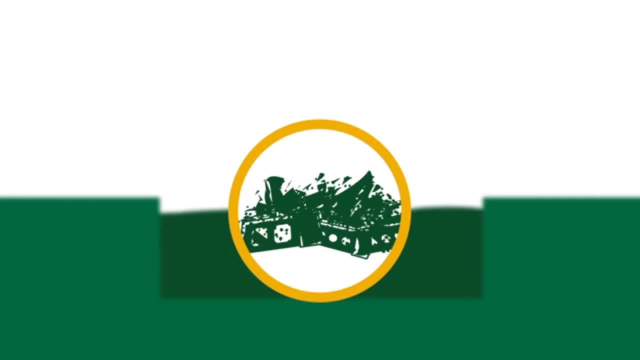 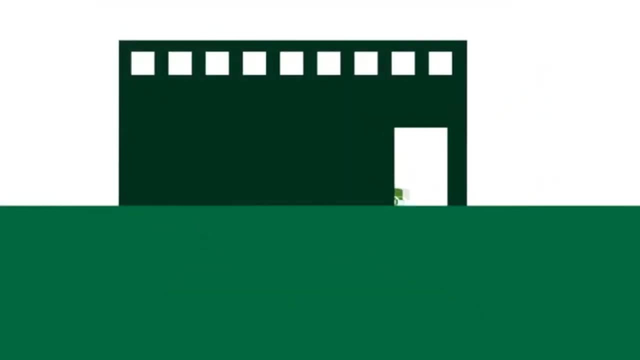 This hazardous treatment methodology is reserved for crushed glass, plastics, bricks, metal shavings and other similar debris types with surfaces that can be completely coated with concrete. The microencapsulation process reduces waste leachability, helping to protect the environment from future exposure. 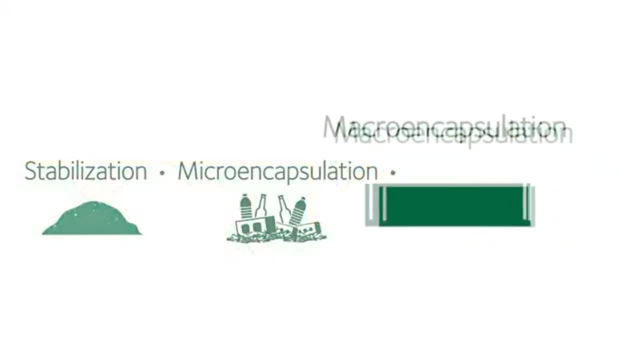 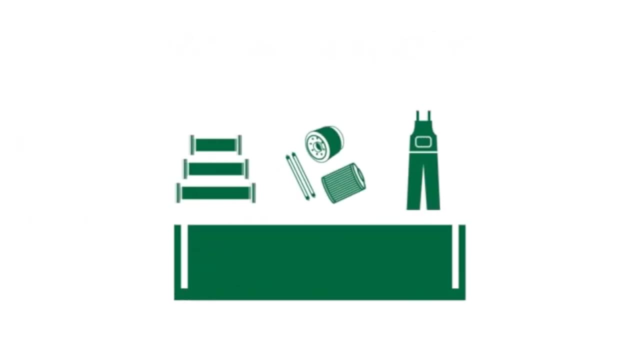 Treated wastes are placed in the landfill. Macroencapsulation is utilized for organic contaminants as well as awkwardly shaped contaminated debris such as clothing, construction equipment and large pipes. These types of items are placed in our proprietary 20 cubic yard roll-off boxes. 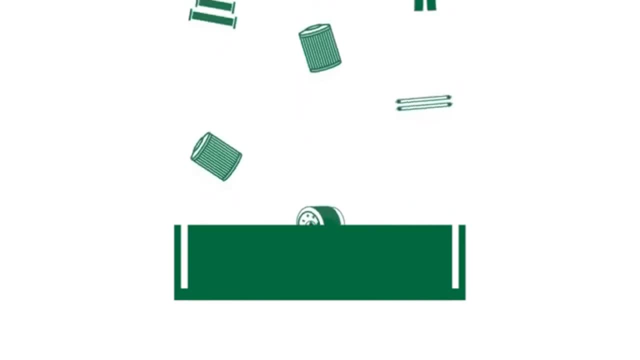 made of high strength, 100 mil. high density polyethylene, until the box reaches maximum capacity. After that, a lid is placed on top and sealed shut. The sealed box is placed in the Subtitle C landfill for safe permanent disposal.